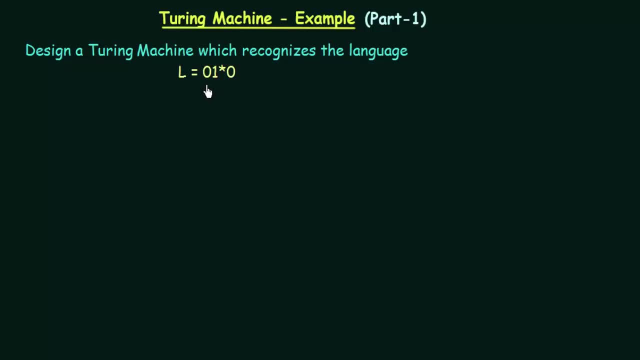 Now, what does this language mean? This language means it should have 1: 0 followed by any number of 1s, followed by 1: 0 at the end. So if you see that this language is a regular language- we might have taken this example even in our previous lectures and you must be knowing that this is a regular language- 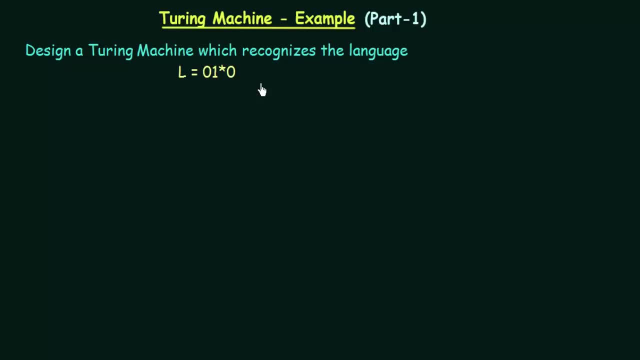 And we actually can design this language using a finite state machine, because this is a regular language. But we are going to do it using Turing machine so that we can understand step by step from the very simplest example of how to design a Turing machine. We don't actually need the full power of Turing machine in order to design this language. 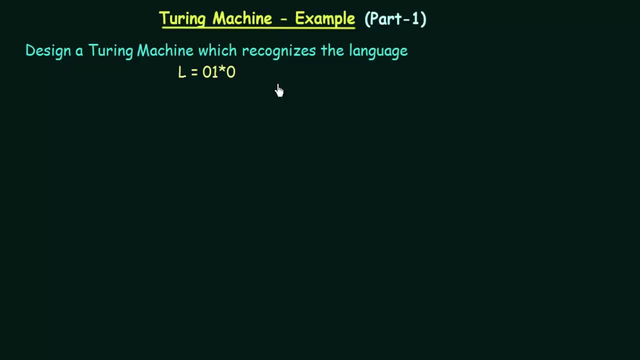 This can also be done with the finite state machine or a push on automata, But we are going to design it using a Turing machine to show you how it actually works from the very basic or simplest steps. Alright, now we are done with the basic or the very simplest steps. 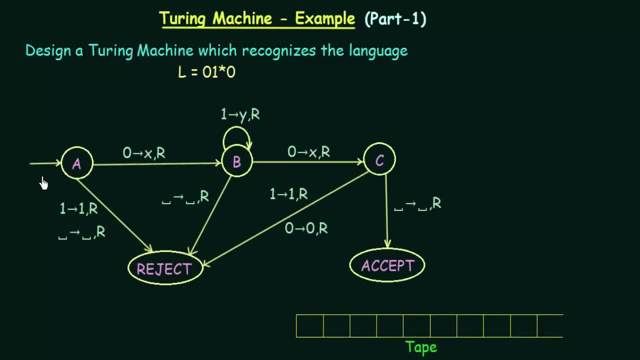 Alright, so we have reached the end of this video. Alright, so we are done with the basic, or the very simplest steps. Alright, so let's see how the Turing machine for this can be designed. So here we have the Turing machine for the language that we have to design, which is L equal to 0. 1 star: 0. 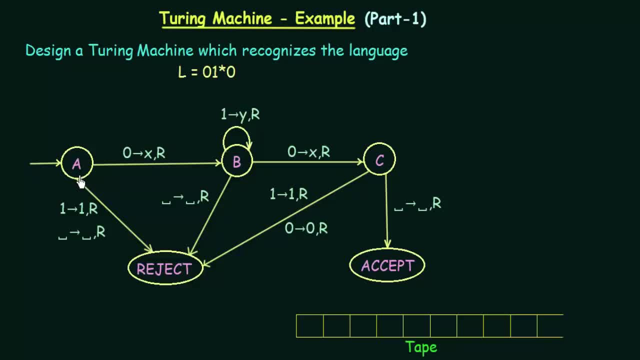 So here we have the starting state, which is A, and then we have two states, B and C, And then we have two final states, which are the reject state and the accept state. And let us see how it works. So, as we want to accept 0, 1 star 0 in the initial state or the starting state, 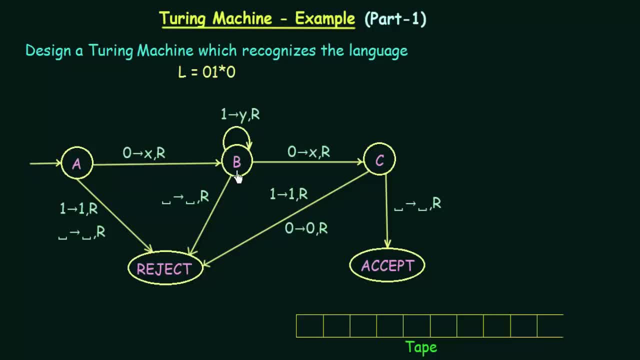 when we get a zero we go to the next state B and then in our tape we write the symbol x and we move right on our tape And we come to state B and we know that we have to accept any number of 1s after we accepted the 0.. 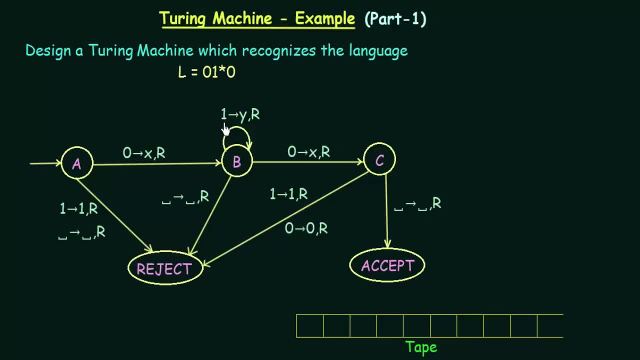 So in state B, if you get any number of ones, you always stay in state B. So in state B, if you get any number of ones, you always stay in state B. you always stay in state B, B. and then in our tape you write the symbol Y and then you move right on the. 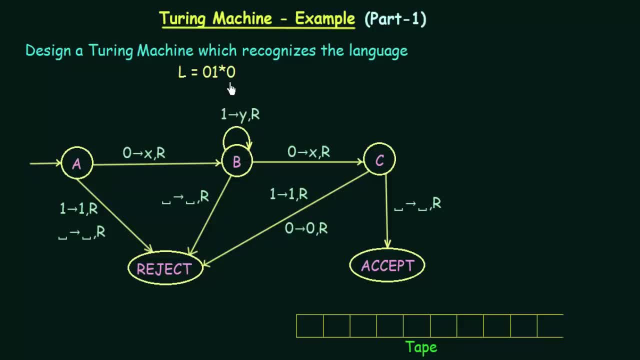 tape, and after getting any number of ones. finally, we need to get a zero. so if you get a zero, what you do? you proceed to the next state, which is state C, and then you write X on the tape and then you move right on the tape and after we 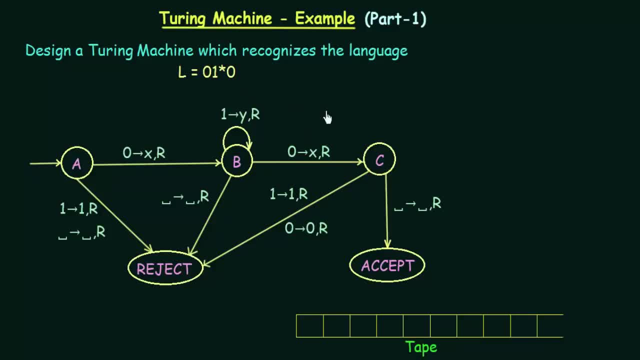 reach the state C, we see that there is nothing more to take. so what we do? we read the blank symbol. that means we read something that is empty or the blank. and if we see the blank symbol, what we do? we don't write any other symbol other than 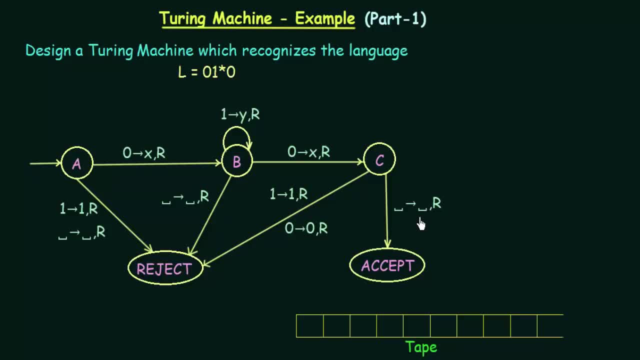 the blank symbol into the tape and then we move right on the tape and it goes to the accept state. so this is how it works. so let us just take an example and see how this works using the tape. so let's say that we are going to take this string 0, 1, 1, 0, so we see that there is 0 and then 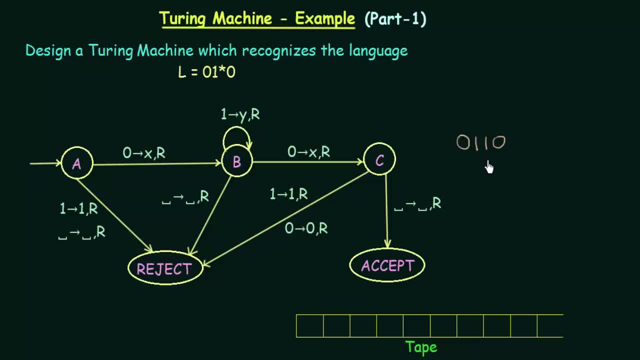 we are allowed to take any number of ones. so we have two ones here and we have a 0 at the end. so this should be accepted by this Turing machine. so first of all we come to the tape, and my tape head is over here in the beginning, and 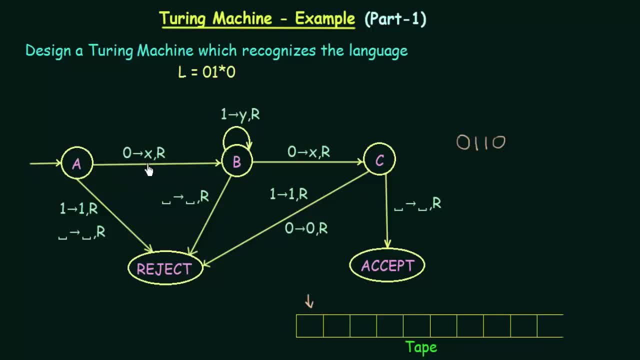 then if you get 0, what happens? we write X on our tape. so in my tape let me write X, and then you go to state B and you move right on the tape. that means my tape head comes over here. now, all right, and now the next input. we have already read: 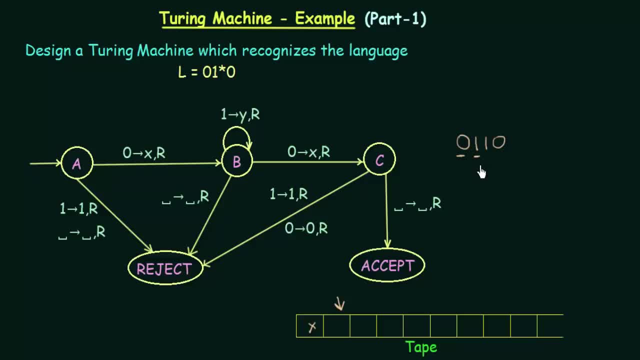 0 and the next input that we have is 1. now, if we get 1, what happens? we are in state B and in state B if we get 1, we stay in B itself and we write Y onto our tape. so this is my tape head. so here I write Y and then what we do. we 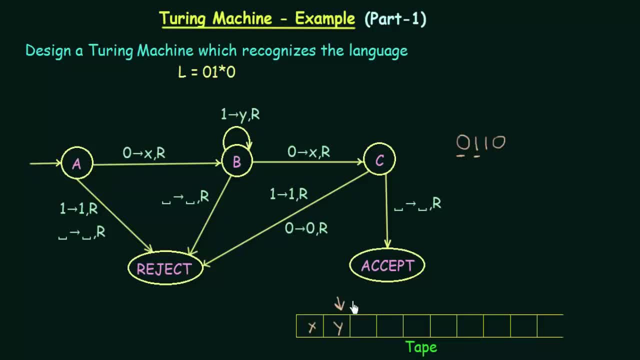 move right on the tape. so my tape head, which was here, we'll now move to the right, which is one step right, alright, and then the next input that we have is another one. so we are still in state B and if you get another one, what you do? 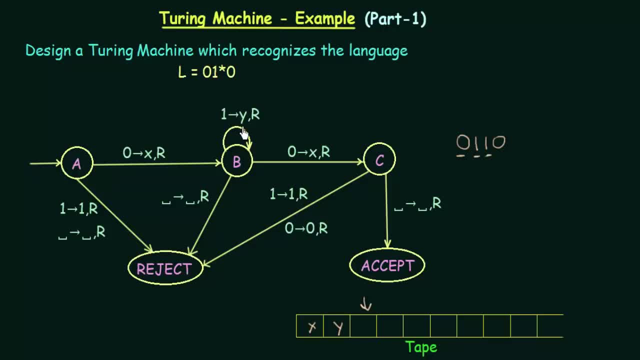 you stay in state B and you write Y on the tape and then you move right. so my tape head is over here, I write Y over here and then my tape head will move one step to the right, which is over here. Okay, and then the next input that I have is a zero. So in B, if you get a zero, what happens? it goes to state C. 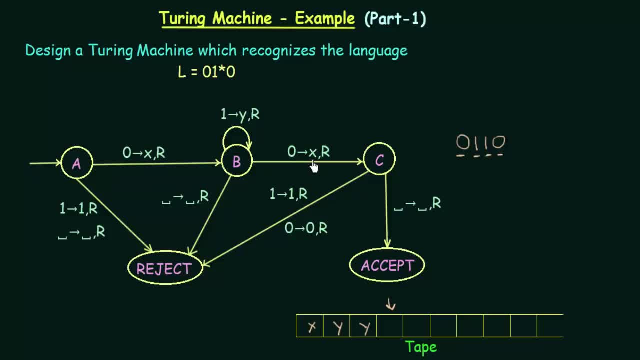 And then we write X on our tape and we move one step right. So I will write X on my tape. My tape head is over here, So just below that I write X, and then we have to move one step right. this right over here. So I move one step right and now we see that we have reached the end of the string. 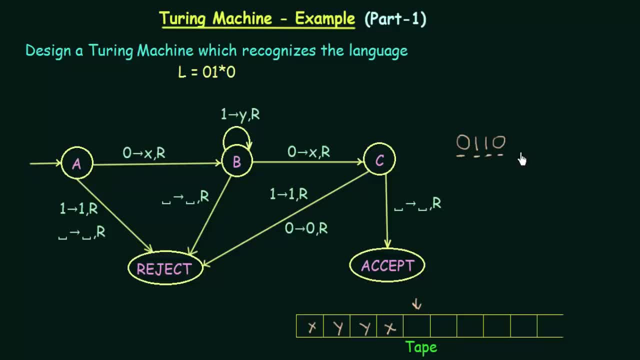 So here there is nothing and we consider this to be the blank symbol. So we are in state C and when we read the blank symbol, what happens? We write blank on the tape and we move one step to the right and we go to the accept state. 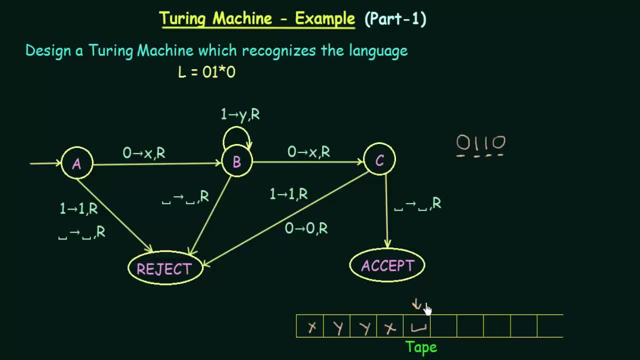 So here is my tape head. I will write the blank symbol and I will move my tape head one step to the right. Okay, so this is the condition of my tape now, and then I have reached the accept state. So, since we have reached the accept state, 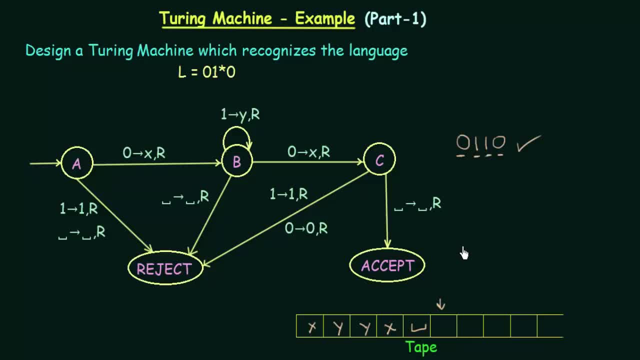 This string will move. This string will be accepted. So this is how the strings will be accepted or recognized by the Turing machine. Now there is one question that you can ask: Why are we writing these symbols- X, Y, Y, X- on the tape? So, as I told you in the beginning, this is a very simple language. 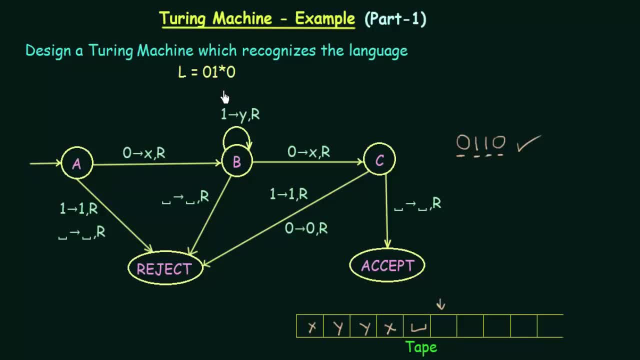 It is a regular language and you actually do not need the full power of a Turing machine in order to implement this, but we have to do this because we are using the Turing machine and, and particularly for this language, this tape symbols don't have any particular use. 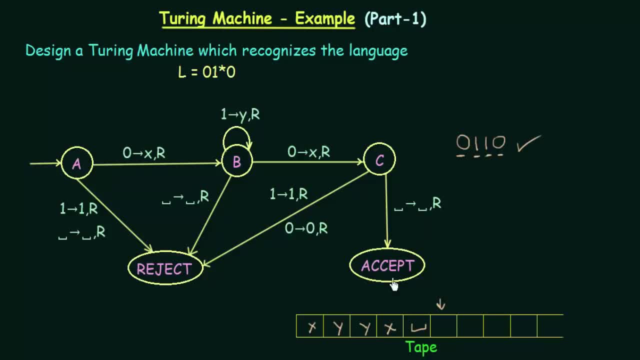 They are not of any particular use for accepting this language, but we are just doing this in order to show you how Turing machine works and how the tape actually works. So you don't actually need the tape, but we have to use the tape because it is a Turing machine. 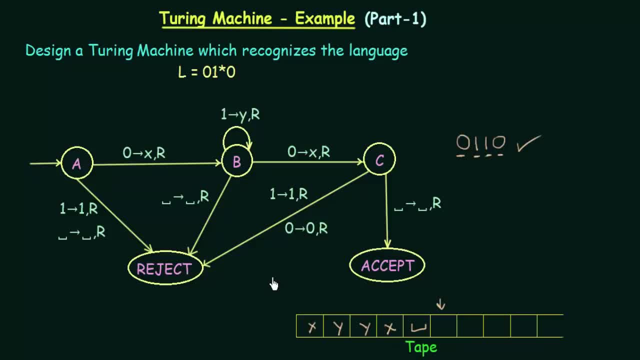 and another thing that you need to know is that in the first lecture itself, I told you that Turing machines, they are deterministic. Deterministic means, when you draw the transition diagram, there should be a transition for each and every input symbol that we have, for each and every state. 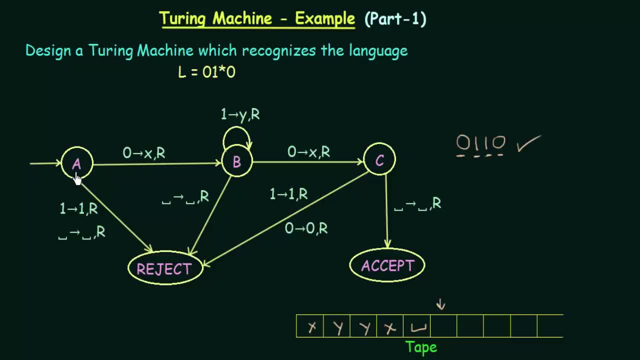 Let's see if this is deterministic or not. Here we have state A and then, in this language, the input symbols that we have. they are 0 and 1.. And the special symbol that we have, which is the blank symbol, that is this one. 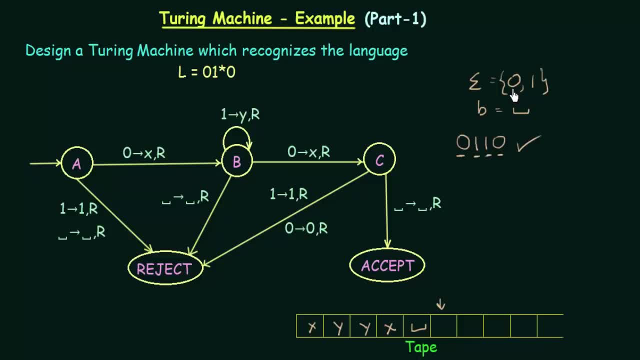 So we need to have transition for the symbols 0 and 1, which is the input symbols, and we should also have transition for the blank symbol. So remember that blank is not an input symbol, but it is a special symbol and we need to have transition even for this. 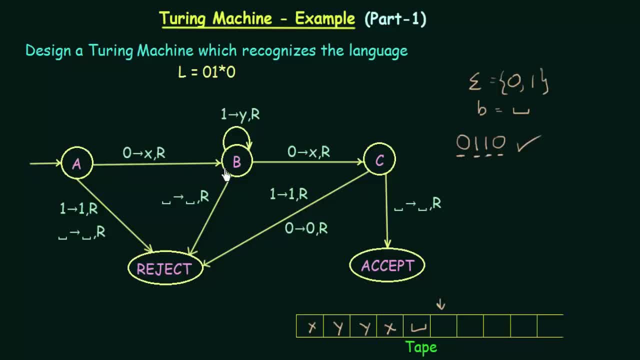 So in state A we see that on 0 it goes to B and on 1 it goes to reject and on the blank also it goes to reject. So for all the three it is having transitions. And even in B, in 0 it goes to C, in 1 it goes to B itself and on the blank it goes to the reject state. 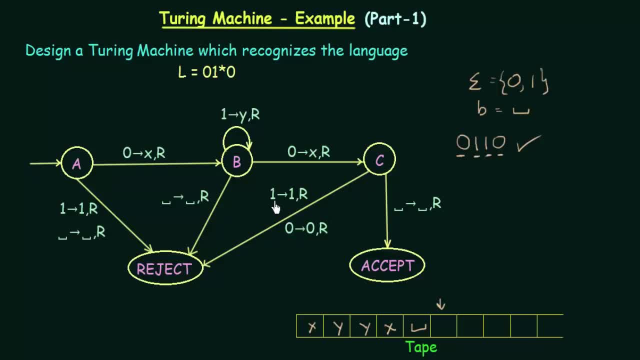 So even in C we see that for both 0 and 1 it goes to the reject state and on blank it goes to the accept state. So we see that for each and every input symbol, including the blank symbol, there is a transition for all the states that we have. 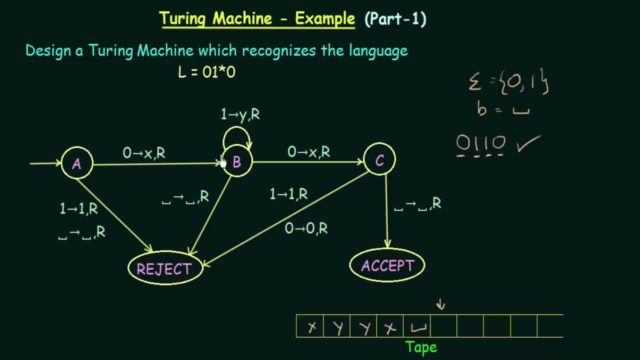 And we see how the student machine was working. For 0 followed by any number of 1's followed by 0, it comes to the accept state. So in all other cases, like if you are getting 1 in the beginning or blank in the beginning, it goes to the reject. 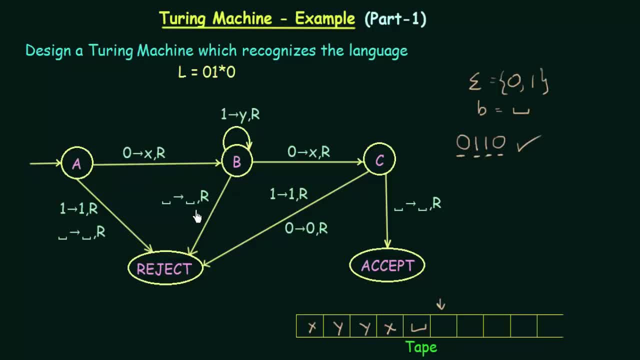 And after getting a 0 in the beginning, if you are getting a blank, then it is going to the reject state And also in C, after getting this 0, which is this final 0 over here And after this, instead of getting a blank, if you are going to get 1 or 0. 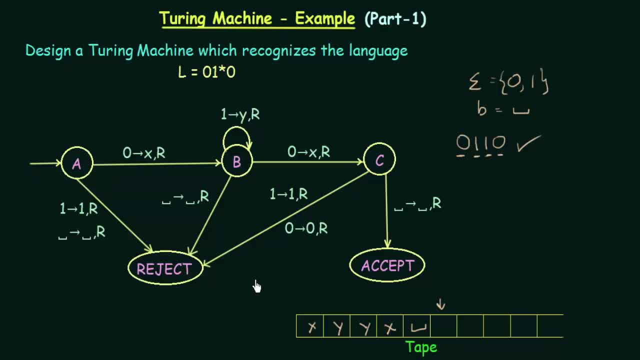 It will also go to the reject state. So this is how this student machine works. And another thing you need to remember about the Turing machine is that sometimes when we draw the Turing machine, you may notice that some edges may be missing. So if some edges may be missing, then you should understand that that edge, by default, it leads to the reject state.